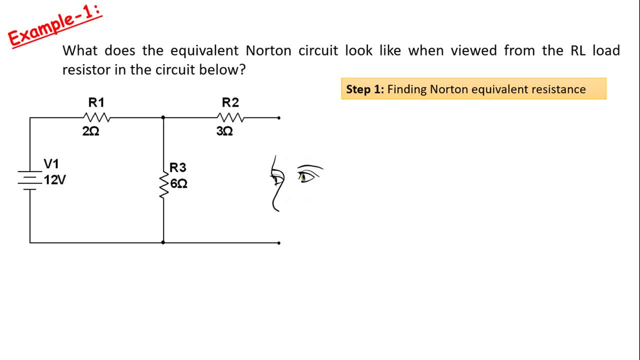 Then we need to open circuit the current sources and short circuit the voltage sources. Since there is only one voltage source here at 12 volts, we need to short circuit it. Now we can find the Norton equivalent resistance Here. R1 and R3 resistors are in parallel. Resistance R2 is connected in series with them. 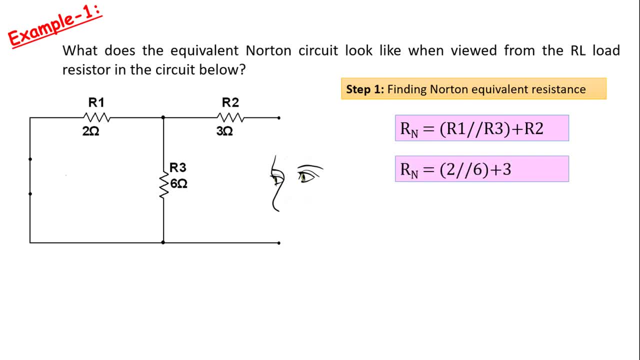 We can write this mathematically as in this formula: 2 ohms and 6 ohms are parallel to each other and 3 ohms is in series. Since 2 ohms and 6 ohms are parallel, their equivalent will be 1.5 ohms. If we add this with 3 ohms in series, 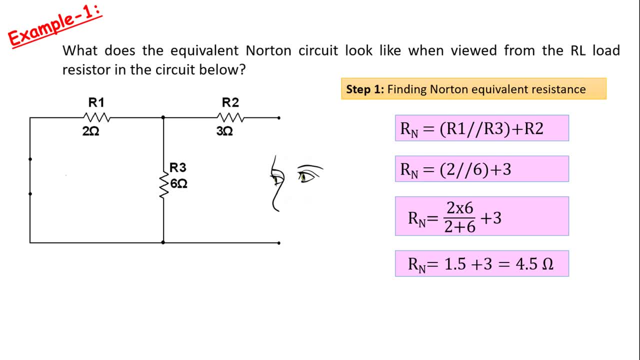 we find the Norton equivalent resistance as 4.5 ohms. Step 2 is to find the Norton short circuit current. We can find the Norton short circuit current if we find the current here by short circuiting where the RL resistor is. The current here is actually the current flowing through the 3 ohm resistor R2.. 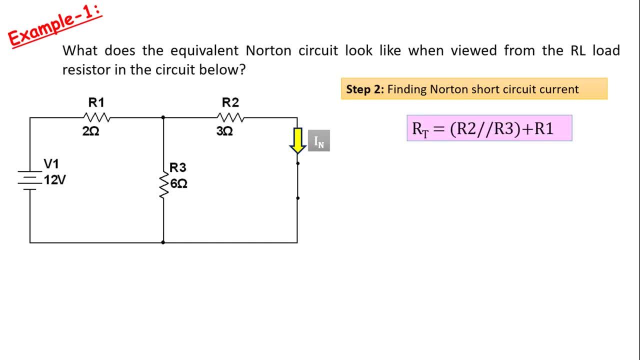 To find this current, we can first find the main branch current. For this we can start by finding the equivalent resistance of the circuit. Resistors R2 and R3 are in parallel. Resistance R1 is in series with them. We can write this mathematically as in this formula: 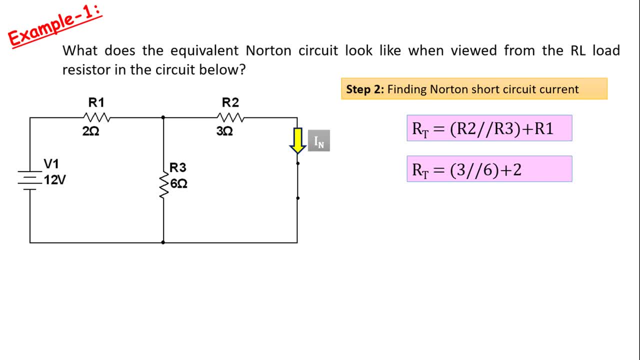 3 ohms and 6 ohms are parallel to each other and 2 ohms is in series. Since 3 ohms and 6 ohms are parallel, their equivalent will be 2 ohms. If we add this with 2 ohms in series, we find the total equivalent resistance as 4 ohms The total. 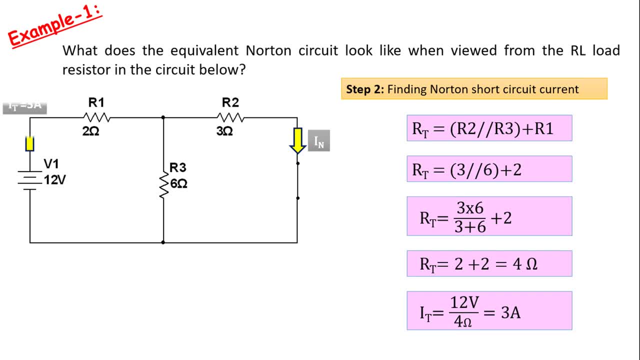 current is 3 amps from 12 volts divided by 4 ohms, The current flowing through the 3 ohm R2 resistor is found as 2 amps from the 3 amps times 6 ohms, over 3 ohms plus 6 ohms formula. 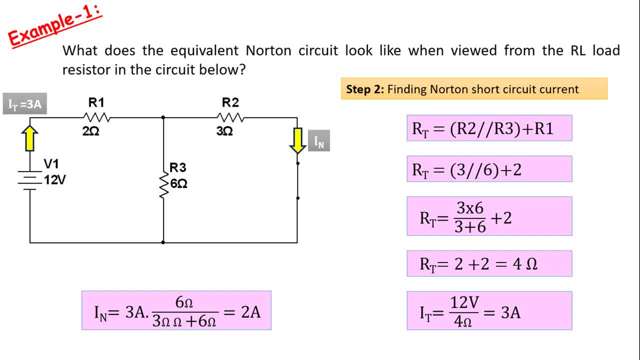 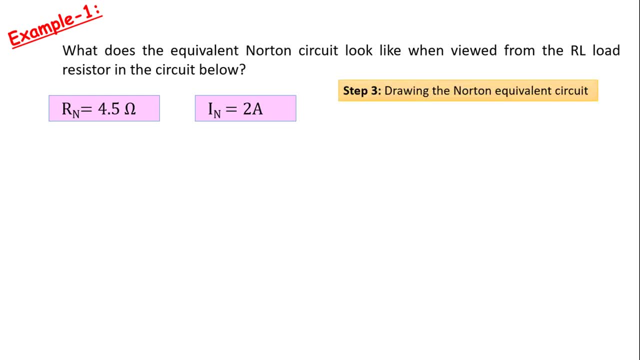 This current is now the Norton short circuit current. We found the Norton equivalent resistance and the Norton short circuit current. The third and last step is to draw the Norton equivalent circuit. The Norton current is shown as an independent current source. The Norton equivalent resistor is connected in parallel to it. We can also connect the load resistor RL to. 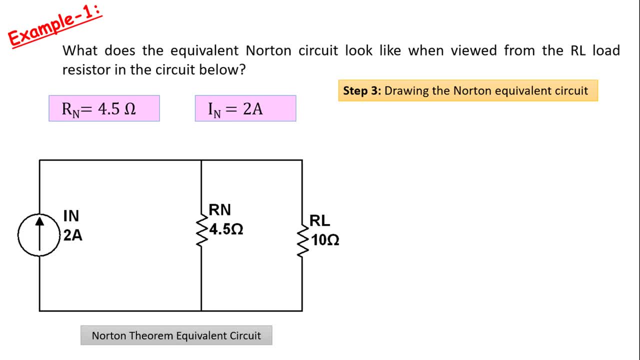 this circuit. From now on you can also find the load current RL if you want. This is the Norton equivalent circuit of the circuit in this example, according to the RL load resistor, If we do source conversion here, that is, if we show this circuit as a voltage source, 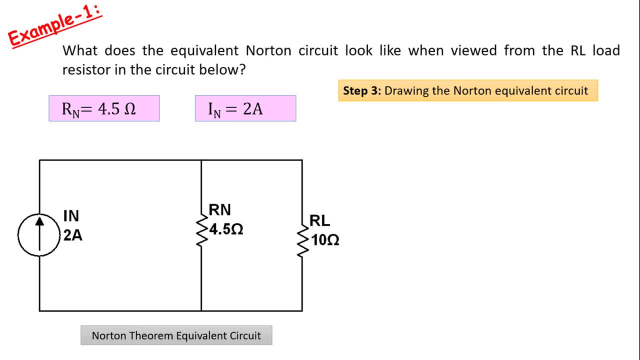 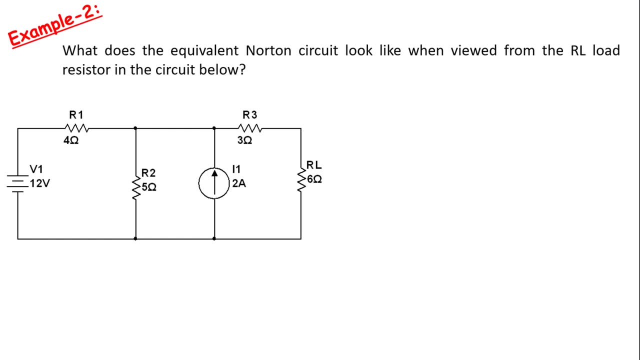 we get the Thevenin equivalent circuit. Let's do one more example for better understanding. Again, in this example let's try to find out how the Norton equivalent circuit is when viewed from the RL load resistance. Again, the first step is to find the Norton equivalent resistance. 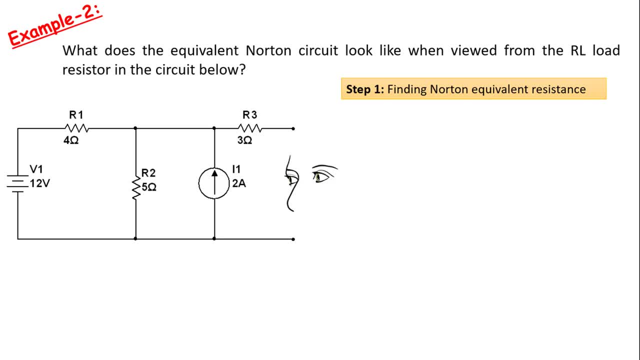 For this we first need to remove the RL load resistor from the circuit where we will look at the circuit. Now we can look at the circuit between these two points. Then we need to open circuit the current sources and short circuit the voltage. 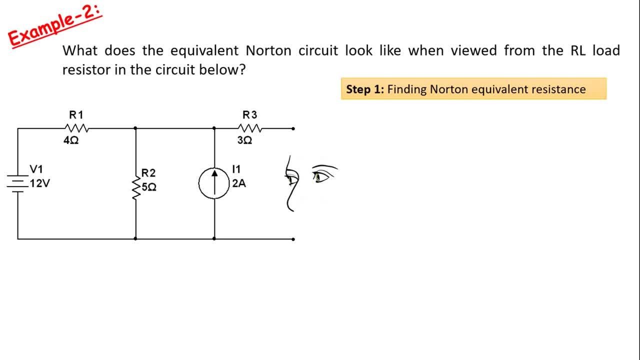 sources. Here we need to short circuit the voltage source of 12 volts and open circuit the current source of 2 amps. Now we can find the Norton equivalent resistance Here. resistors R1 and R2 are in parallel. Resistance R3 is connected in series with them. 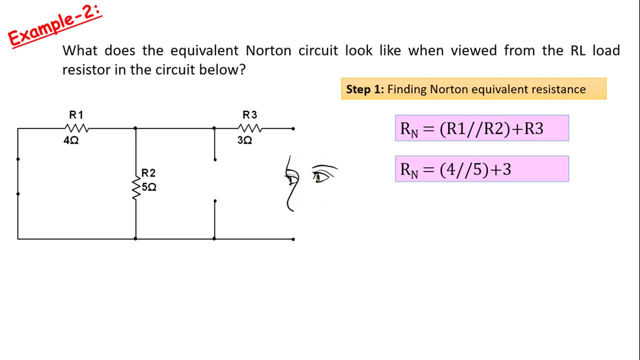 We can write this mathematically as in this formula: 4 ohms and 5 ohms are parallel to each other and 3 ohms is in series. Since 4 ohms and 5 ohms are parallel, the equivalent will be 2.2 ohms. 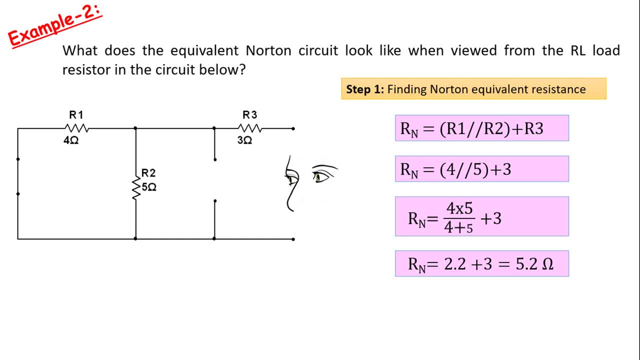 If we add this with 3 ohms in series, we find the Norton equivalent resistance as 5.2 ohms. Step two is to find the Norton short circuit current. We can find the Norton short circuit current if we find the current here. 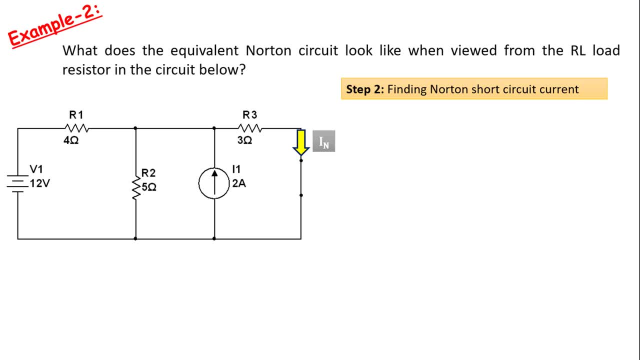 by short-circuiting where the RL resistor is, The current here is actually the current flowing through the 3 ohm resistor R3.. To find this current, if we find the voltage at the point I indicated as Vx IN Norton, current can be found by dividing this voltage by the 3 ohm resistance R3..